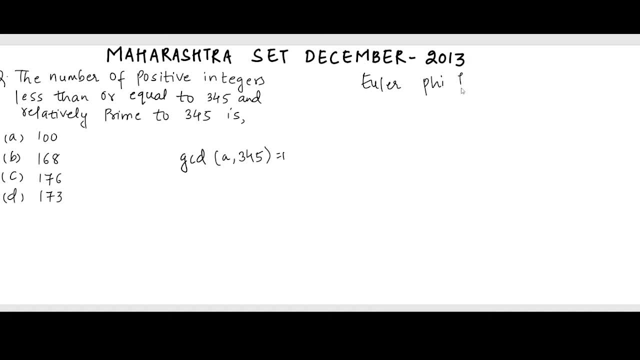 This is based on Euler 5 function. It is set theoretic function. I have made a separate video on this. I will put the link in the description box. You can check that out. There is a dedicated video on this set theoretic function. 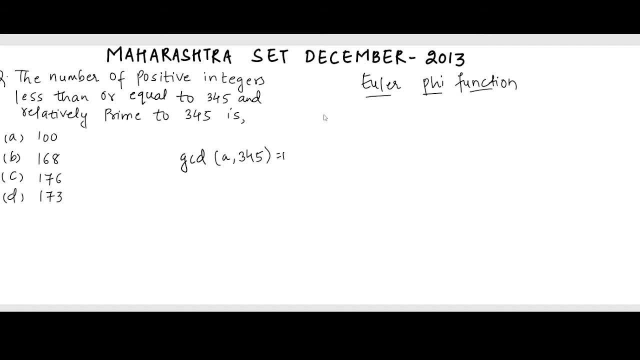 So now let's start. So we will use that and we will directly find the positive numbers of 345, which are less than 345 and relatively prime to 345.. How many numbers are there? So now what we have to do is See the 345 is. 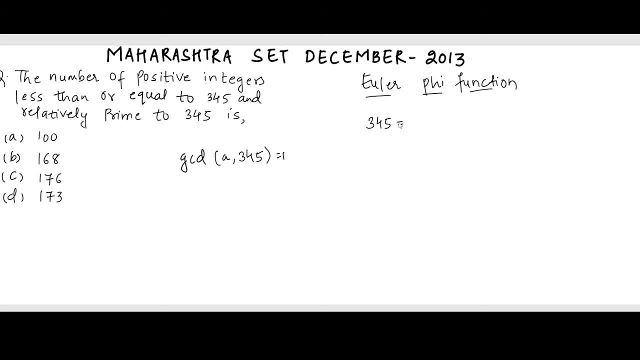 First of all, you take it in prime power factorization. Take out its factors. So what are its factors? 345. Let's find factors of this. So 345 is 345.. Let's find factors of this. Let's find factors of this. 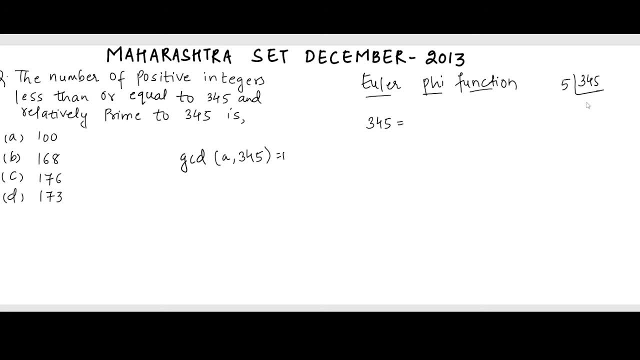 So if we will use table of 5, then how much will it be? This will be 6 and 69. Then again table of 3.. So this is 2 and 3, 23.. So 23 is prime number. 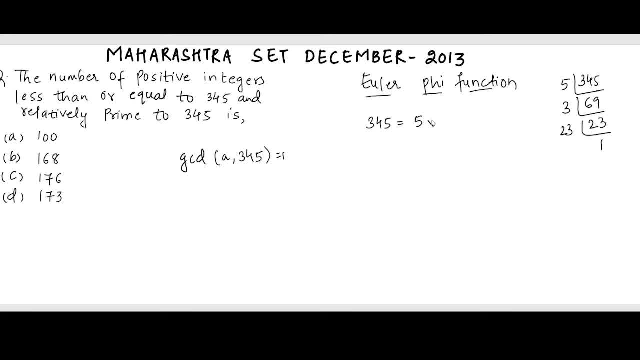 So this will be. So what is its prime power? factorization 5 into 3, into 23.. Okay, So now suppose I have any number in which I have given p1, k1, p2, k3, k2 till. 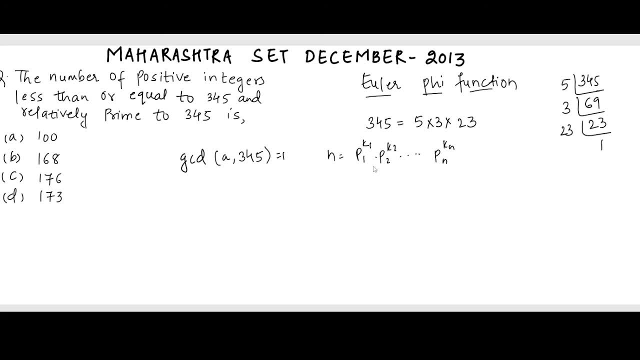 pn kn. If I can write its prime power factorization like this, then what is my phi n? Phi n means the Euler phi function. We denote phi? n as number of positive integers, positive integers which are relatively prime, relatively prime to n and less than n. 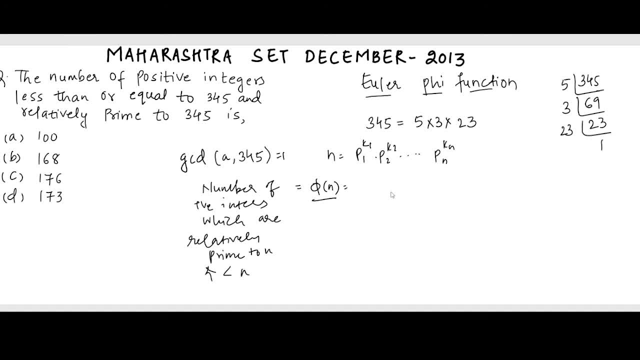 This is also important. We denote it by phi n only. So what is the formula of phi n? p1 raised to k1, into p2, raised to k2, till pn, raised to kn. Then what you will do? 1 minus 1 upon p1. 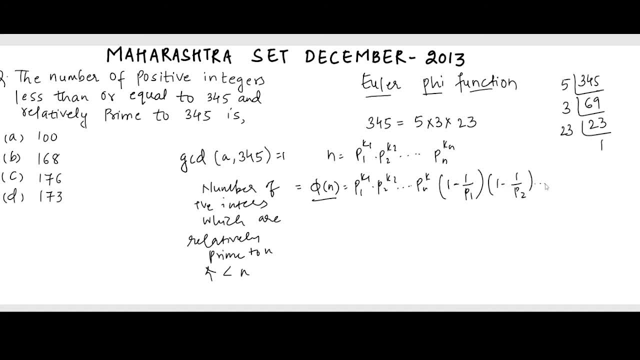 1 minus 1 upon p2, till all the factors here, pn, so 1 minus 1 upon pn. This is the formula. So now we have n, value 345, which we have kept 5 into 3, into 23..